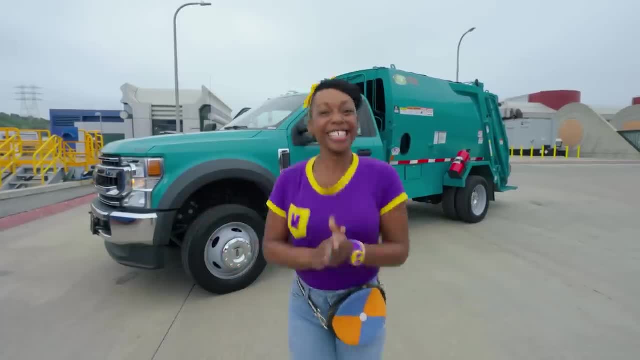 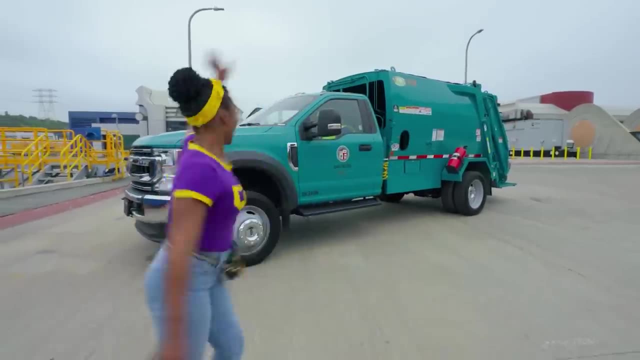 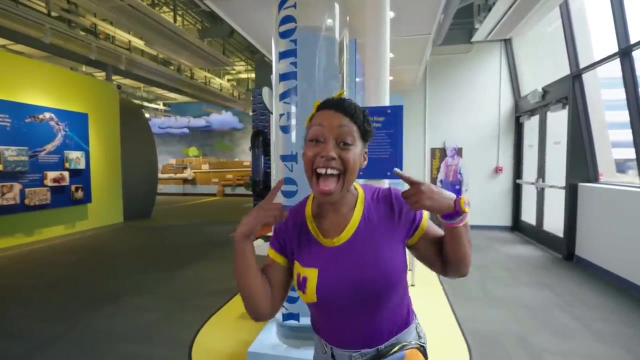 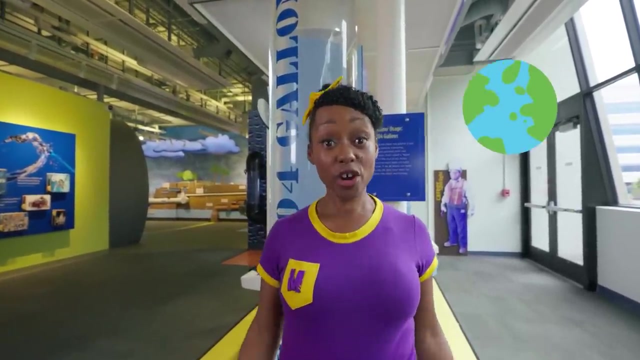 all about recycling. Okay, one, two, three, four. Are you ready to explore? Yeah, let's go. I spy with my Mika eye a glass tube full of water. Did you know? 70% of the Earth's surface. 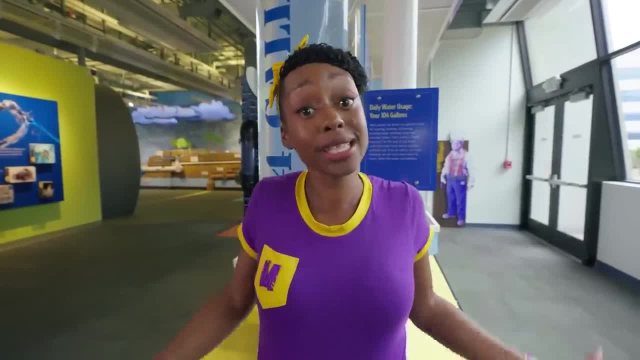 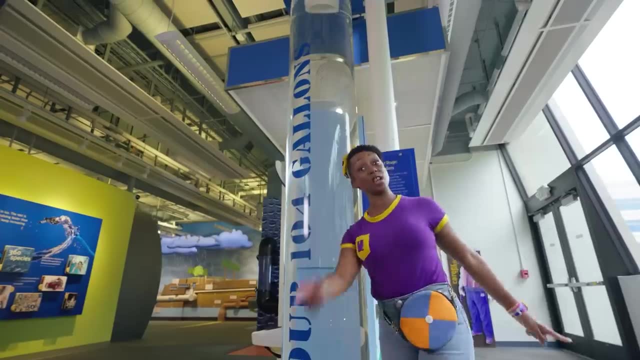 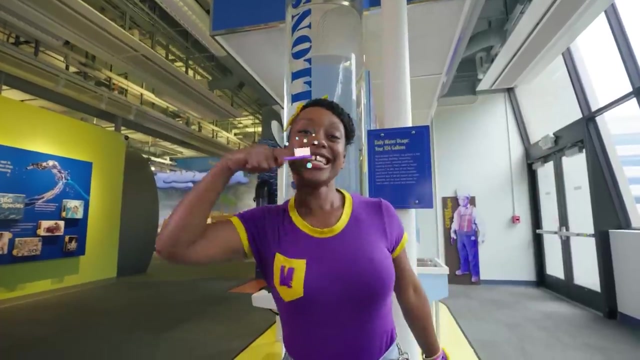 is water, Mm-hmm, but less than 1% of it can be used at home. Whoa, This tube has all the water one person uses in one day to do things like take a shower, brush their teeth and wash their hands. 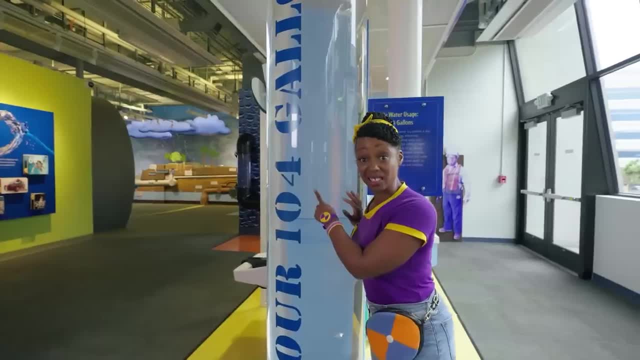 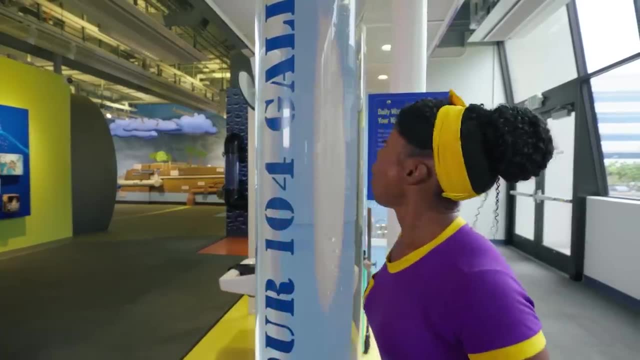 This says 104 gallons Whoa. that's a lot of water. It's about three bathtubs full Whoa Whoa. Hmm, I wonder what I'm going to do, What other things we do with this water. Let's go find out. 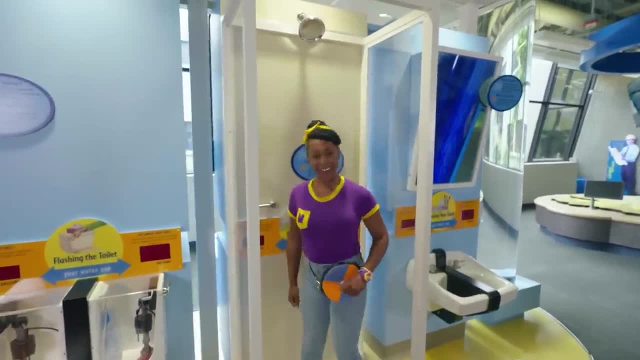 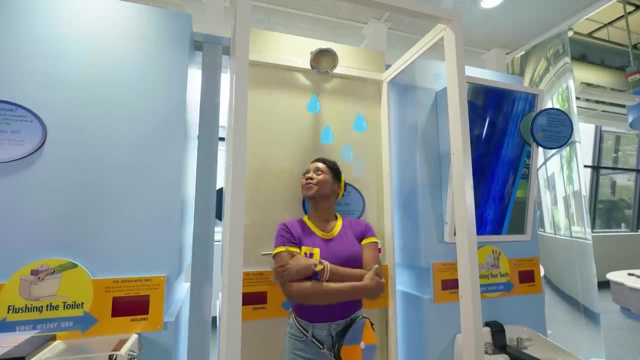 Whoa shower. Okay, time to get clean. Whoa, that water's still chilly. Ah, that's nice. Scrub, scrub, scrub, Le-ha-ha, De-da-da-ha, De-ha-ha. 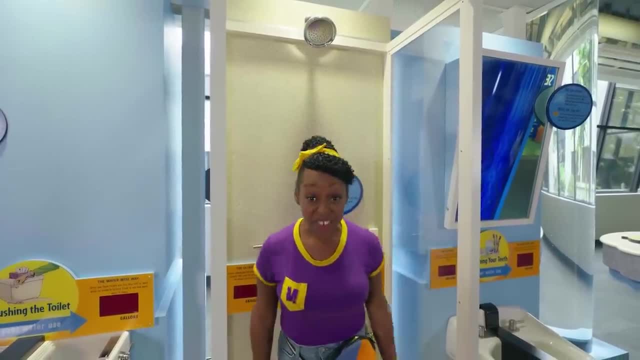 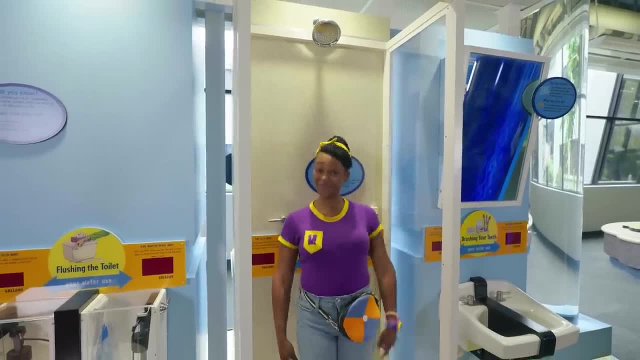 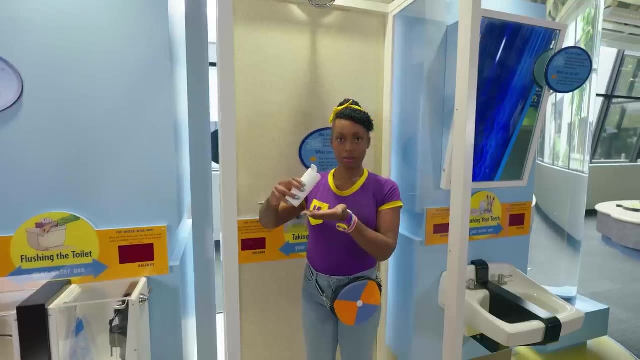 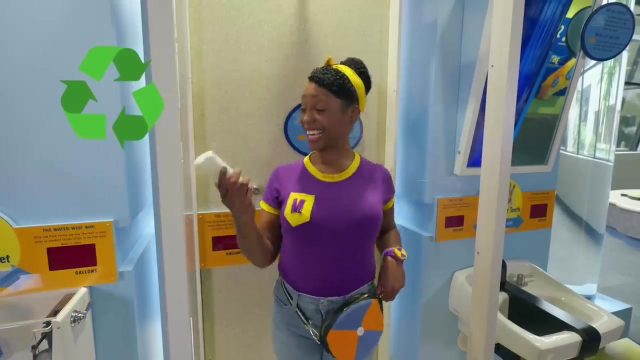 of water by showering for three minutes less. Hey, some shampoo. I'll wash my hair. Huh, it's empty. I know let's save it for later so we can recycle it. It's made out of plastic. I'll put it in my jam pack. 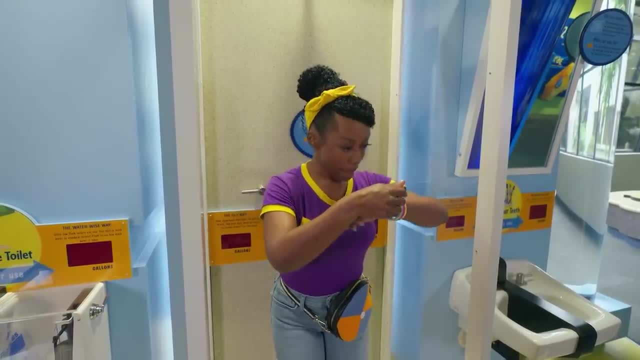 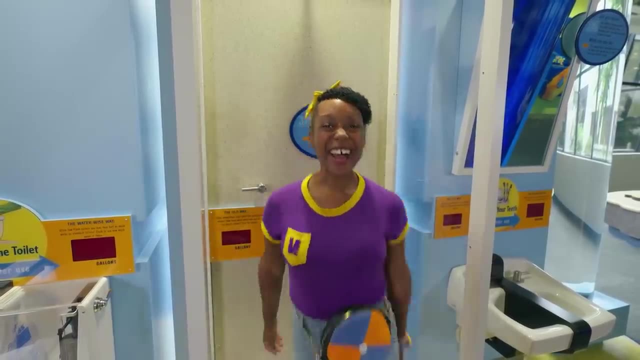 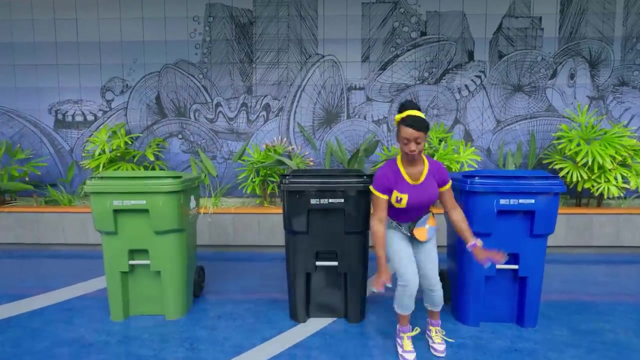 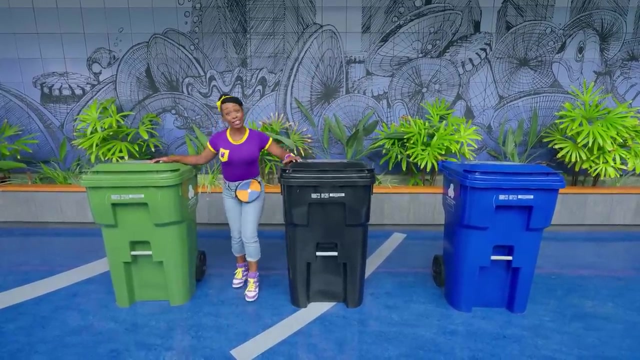 And let's see where we should go next. Huh, my navigator says there's more to see That way, Here we go. Whoa, look at all these colorful bins. The green is for compost, like banana peels and orange peels. 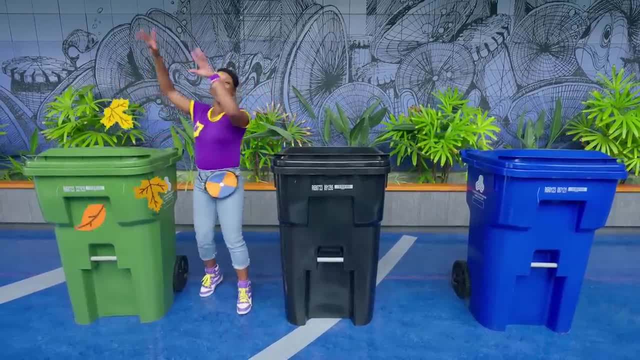 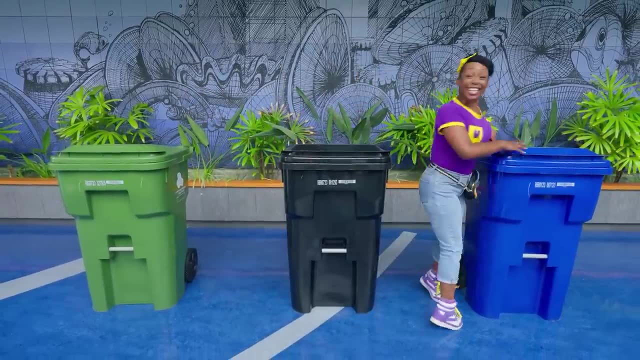 and all sorts of other things, And also yard waste too, like twigs and fall leaves. And the black one is for trash. This can't be recycled. But this blue one is for recycling- For paper, plastic, metal and glass too. 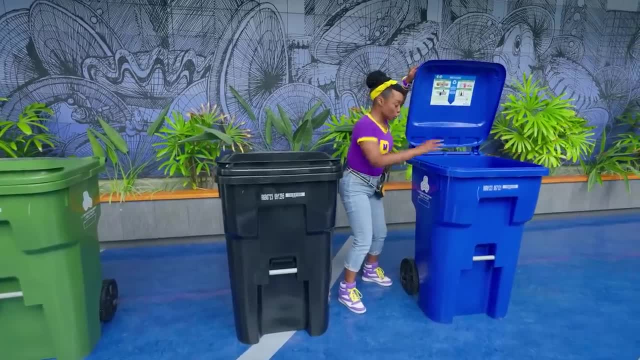 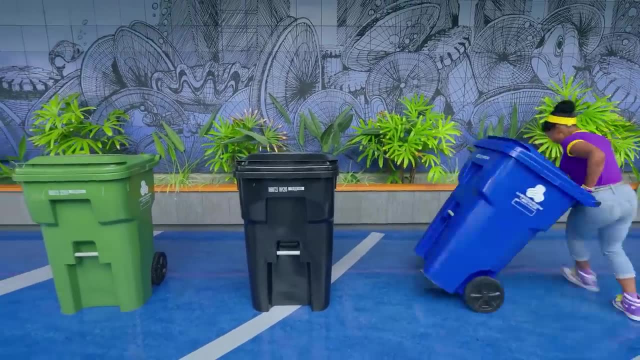 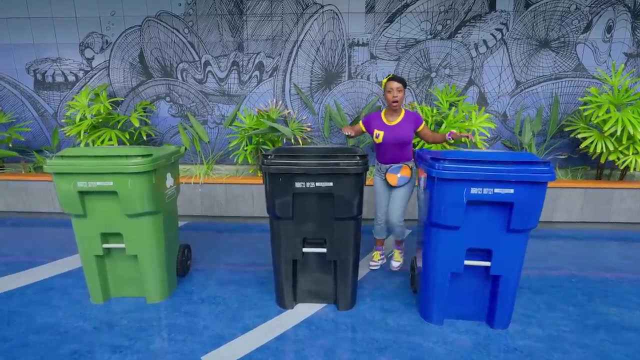 You take all those items, you put them in, shuggle it and then the recycling truck comes and takes it to the recycling center. Woo, Woo, Wait, I know Let's go explore and see if we can find some items to sort. 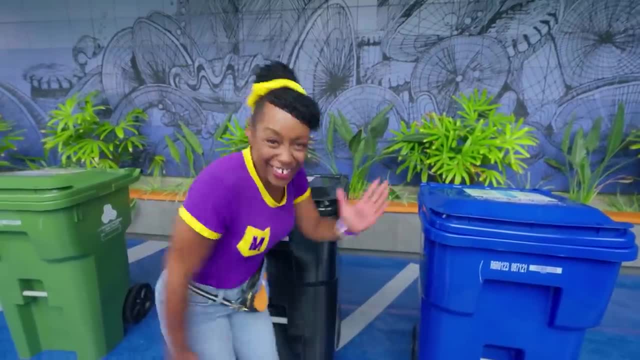 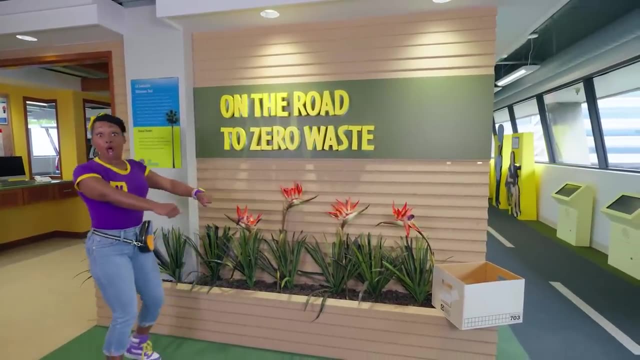 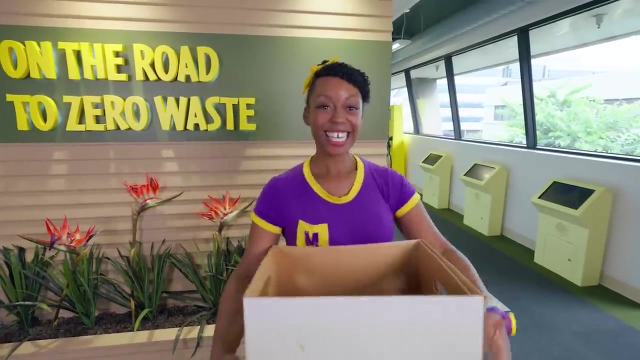 Good idea, huh? Okay, let's go. Woo, I'm on my Mika cycle and I'm on the road to zero waste. Look, There's something we can recycle: A cardboard box. Did you know? cardboard boxes are made out of paper? 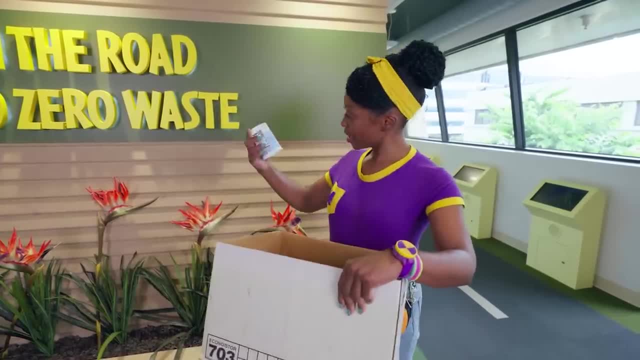 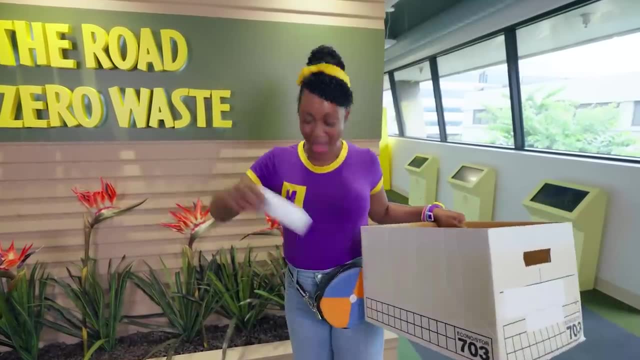 Mm-hmm, And they're recyclable. Oh, and look, There's a plastic cup in here. We can recycle that too. Oh, and I can add my shampoo bottle. Yeah, Let's see what else we can recycle. 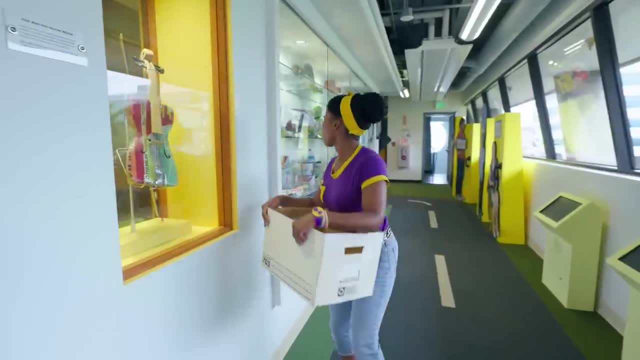 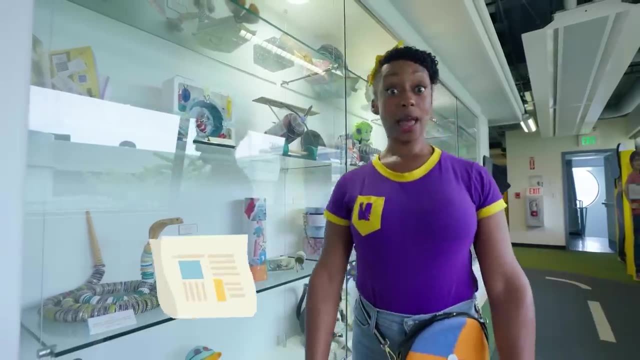 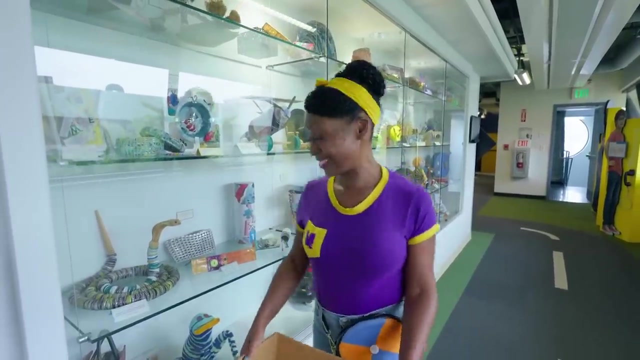 Come on, Whoa, Check out this case. It's filled with things that people made out of- things like paper, glass and plastic, Mm-hmm. Instead of throwing it away, they turned it into things they could use, like this snake. 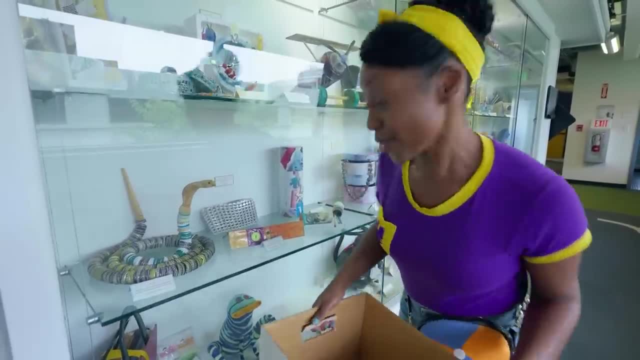 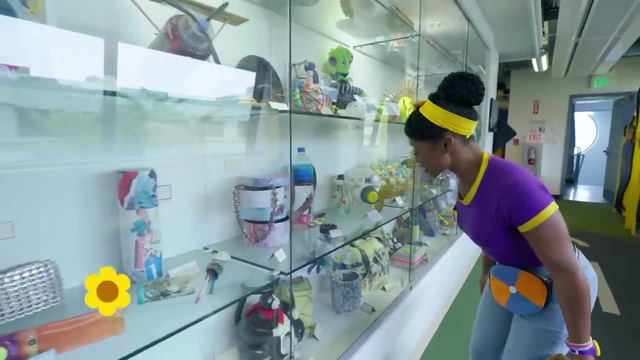 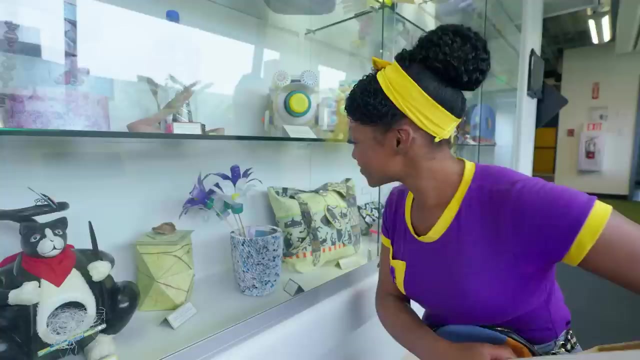 Whoa, It's made out of bottle caps. Wow, So cool. Oh, and look at these flowers. The vase is made out of magazines that have been upcycled And the flowers are made out of bottles. Oh, they smell lovely. 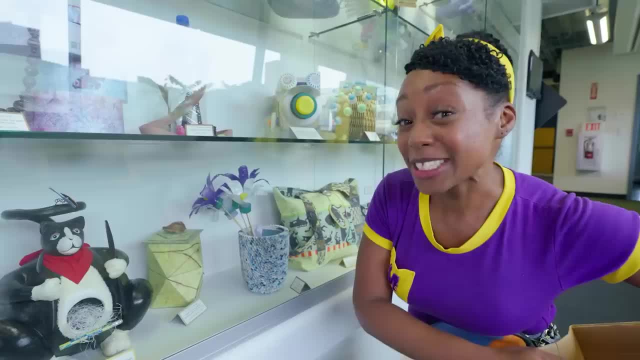 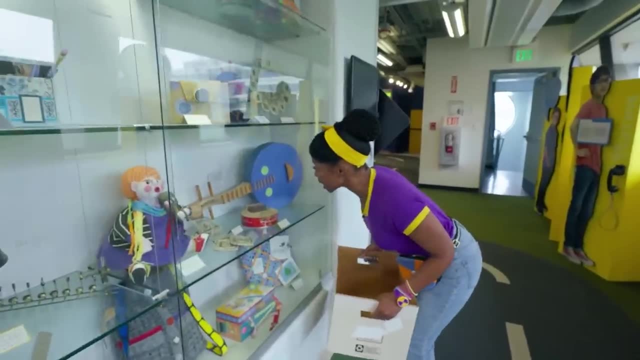 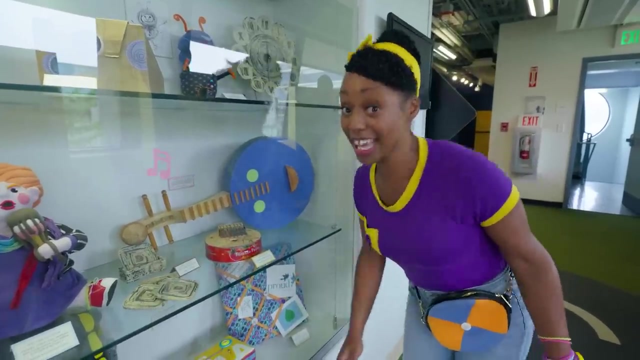 Oh, and they're purple, One of my two favorite colors. Oh, beautiful Whoa, What's that? Look at this cool instrument. It's called a Chinese moon guitar and it's made out of clothespins and cardboard and lots of other materials too. 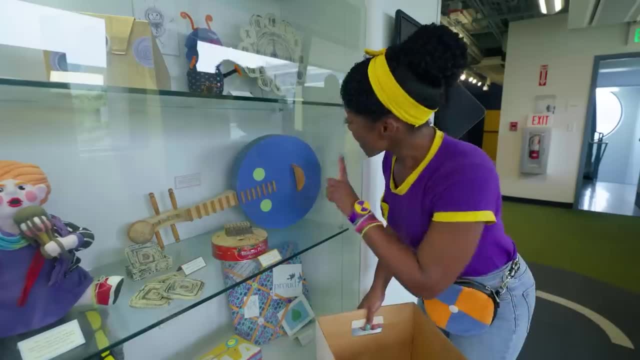 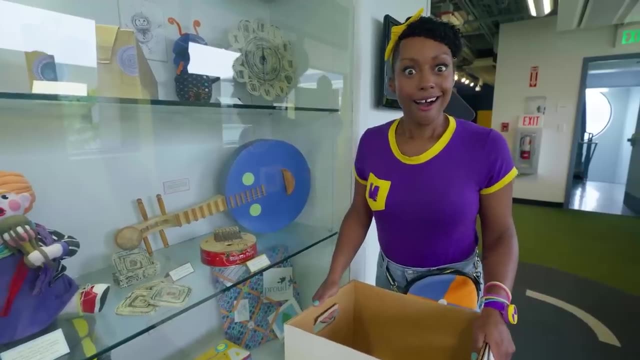 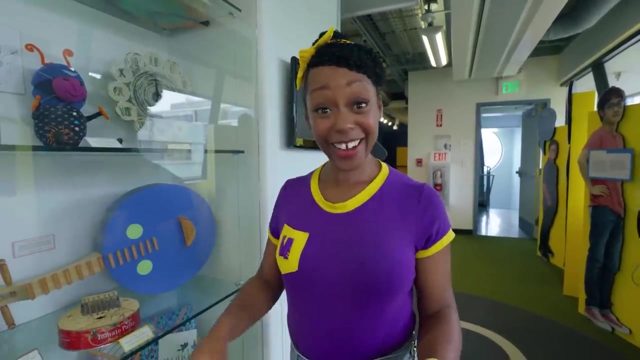 Ooh, The colors kind of remind me of the Earth: Blue, green and brown Boy, I have an idea. Oh, I feel so inspired by these items. in this case, I'm going to reuse something in here to make something new. 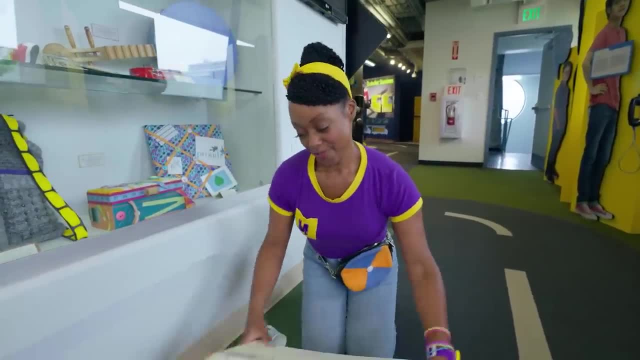 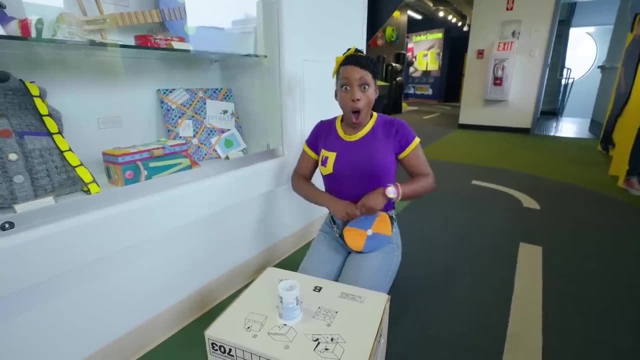 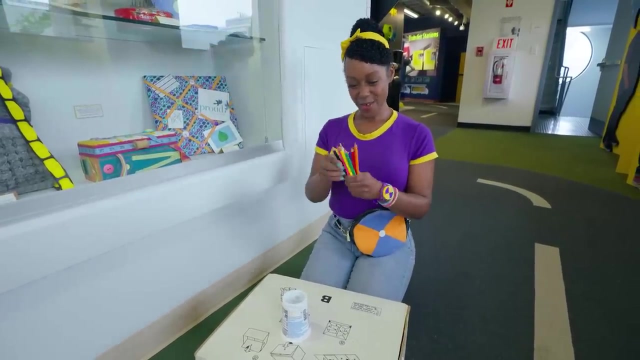 Okay, I'm going to use this box for a little table to make some art. I'll take this plastic cup. Oh, I have some colored pencils in my jam pack. Yeah, it could be a pencil holder. Put the black pencil in and the pink pencil in and the white, yellow, red, green and. 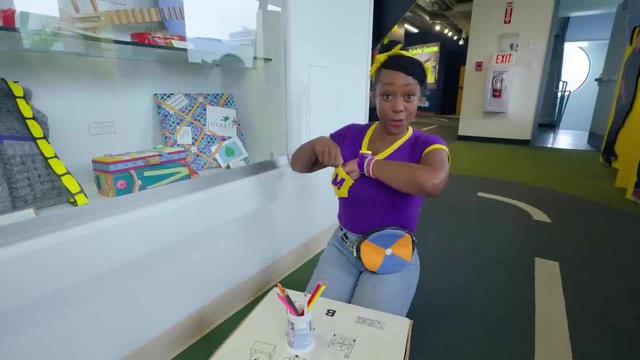 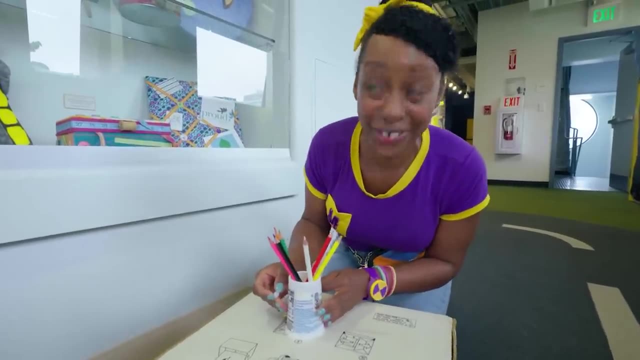 orange. Hey, I have some googly eyes in here and I'll stick them on just to make it extra silly and creative and cute. There we go: One googly, Two googly eyes. Check it out. Wow, It is fun to reuse and recycle. 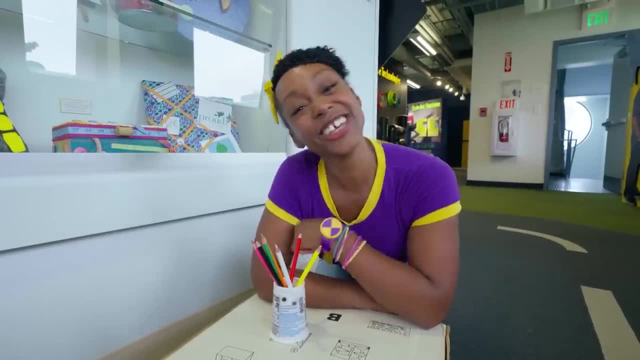 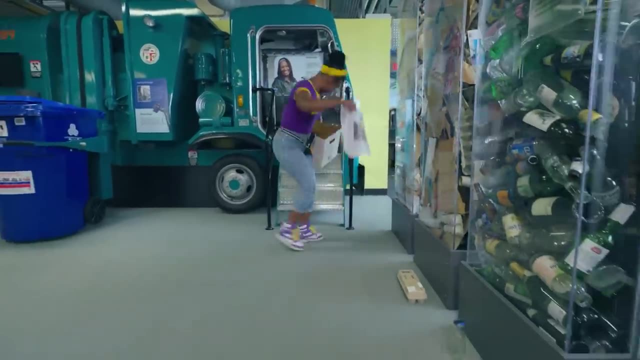 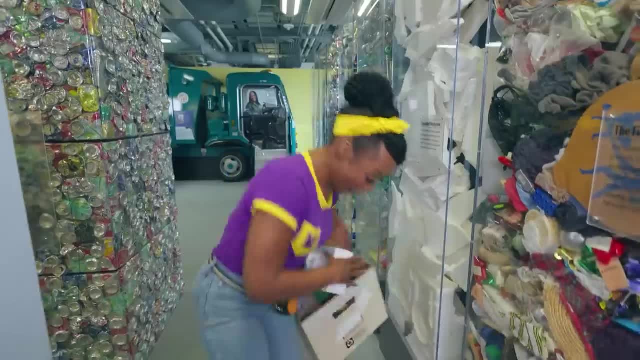 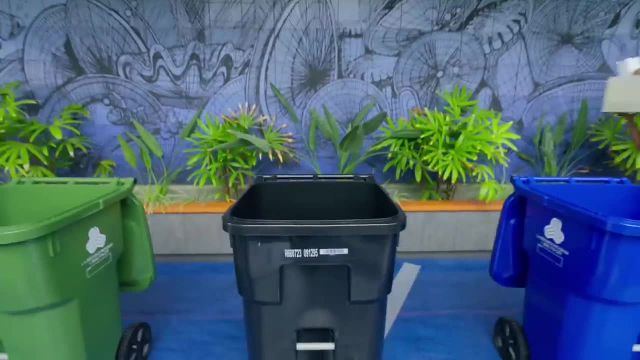 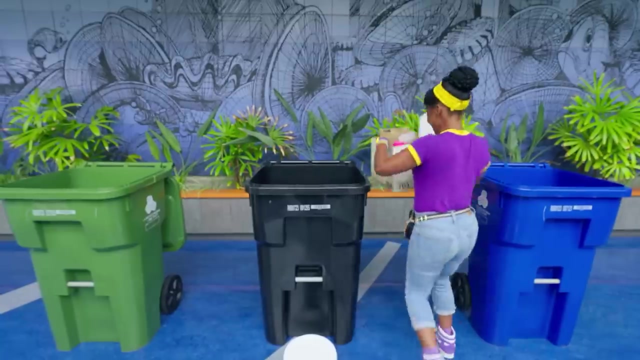 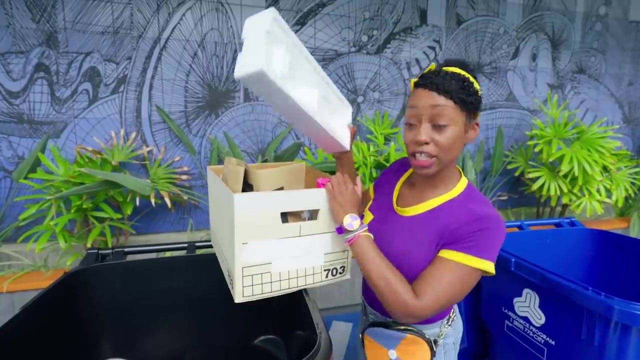 Wow, Now let's go sort these items. Okay, we have our items. Let's play our sorting game, Okay. Okay, let's see Styrofoam. Oh, this might come in the packaging of your toys that are delivered. 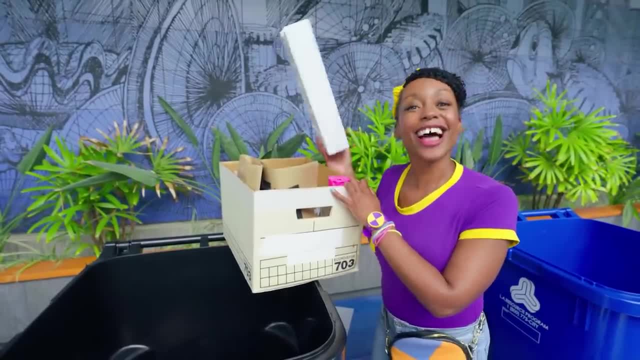 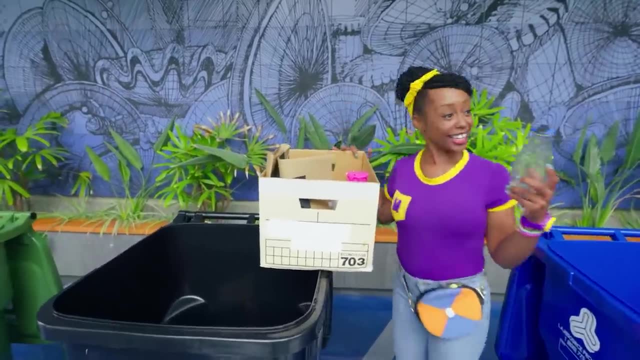 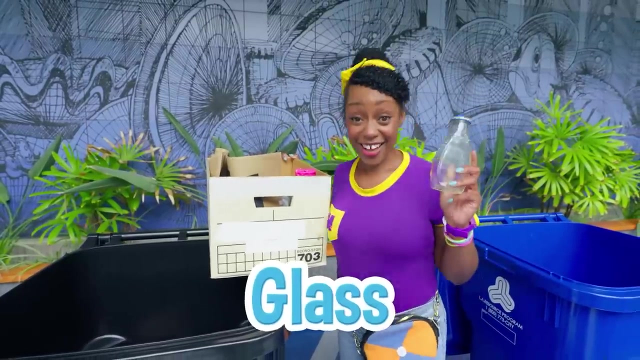 Can this be recycled or is it trash? That's right, It goes in the black bin Trash. Hmm, what about this? Huh, looks like maybe it used to be some juice or some syrup. It's glass. Where does glass go? 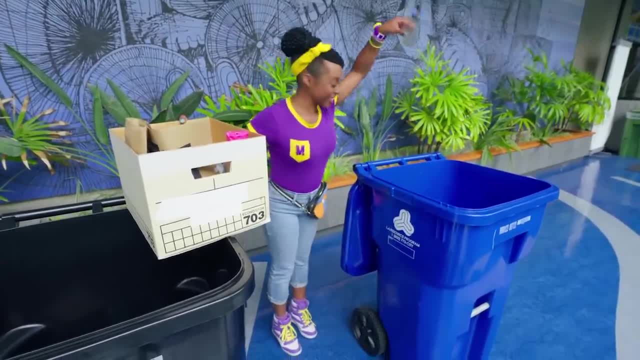 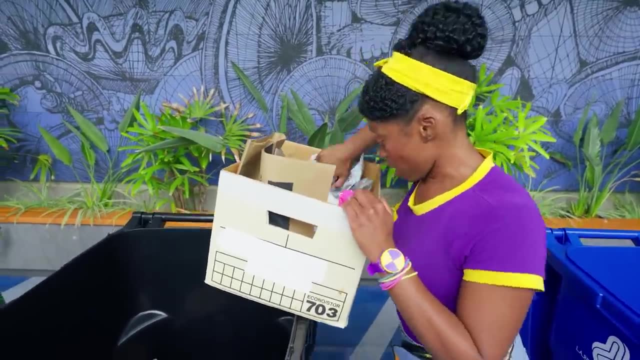 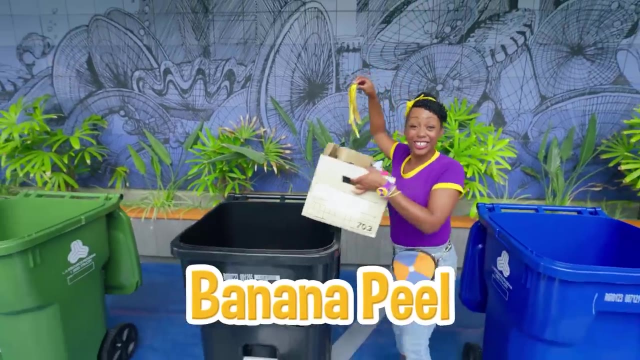 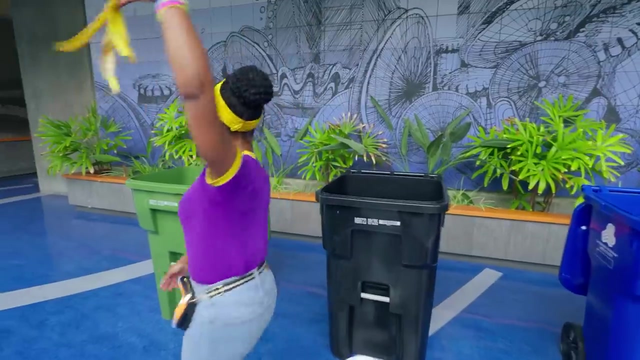 Right Glass can be recycled in the blue bin. Okay, what else is in here? Oh, what about this? A banana peel. Do you know where the banana peel goes? Uh-huh, that's right Into the compost, Woo-hoo. 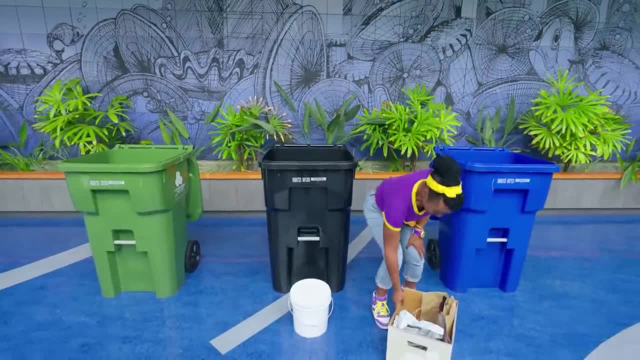 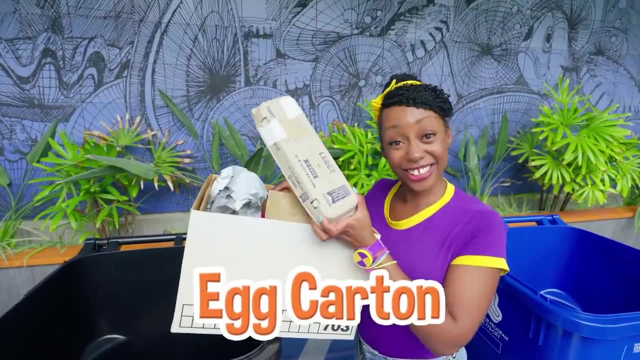 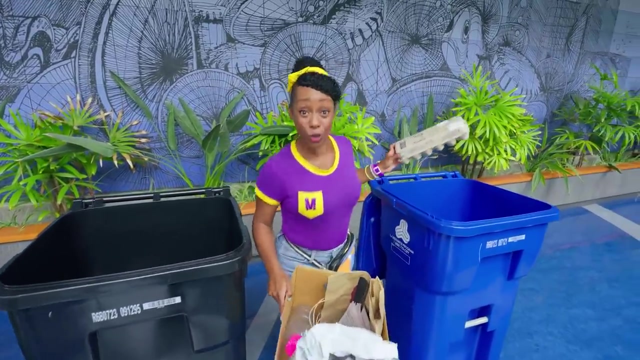 Bananas are delicious. Lots of potatoes, Lots of calcium. Okay, what else? Check it out. Do you know where the egg carton goes? Uh-huh, into the recycling? Did you know a dozen eggs is 12 eggs? 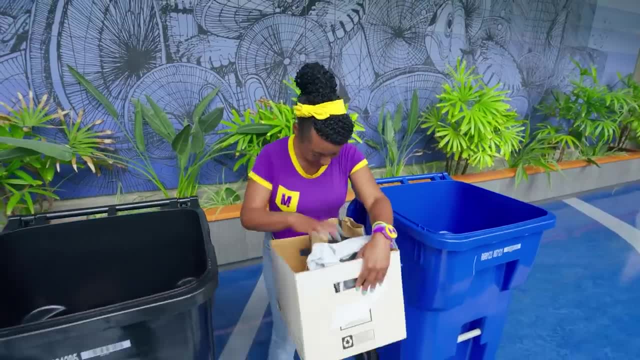 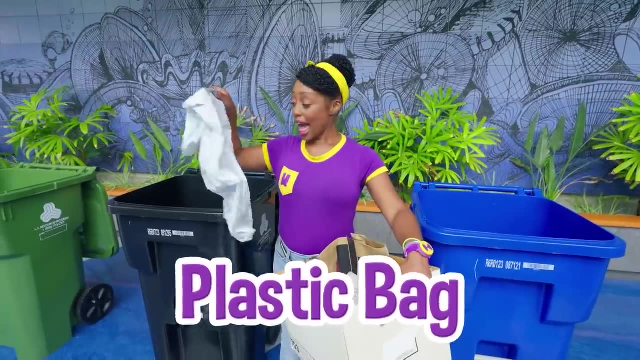 Oh yeah, There you go, See you later. Ooh, what about this? This is a plastic bag. Looks like it had a delivery with lots of stuff. Looks like it had a delivery with lots of stuff: Lots of toys and cool things to play with. 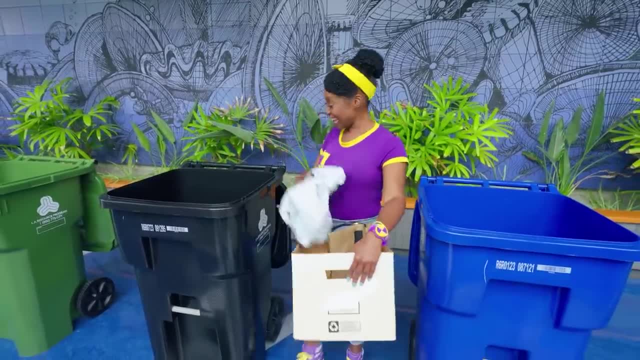 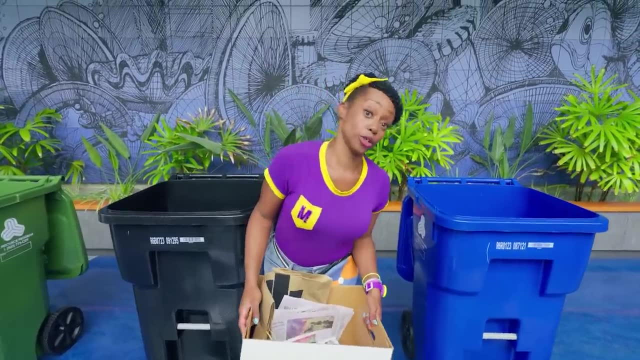 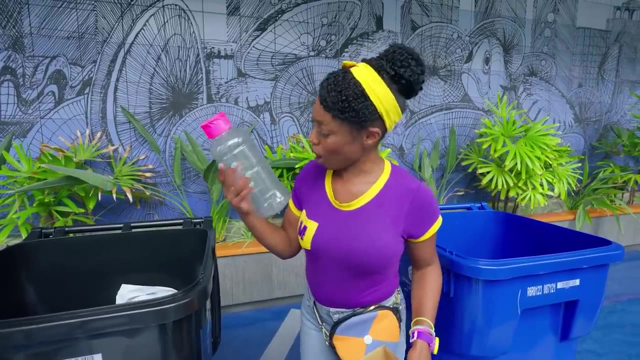 Do you know where it goes? That is right Into the trash, Because, even though it's plastic, only certain types of plastics can go into recycling. Oh, like this one, Hard plastic can be recycled. Ooh, I wonder what used to be in here. 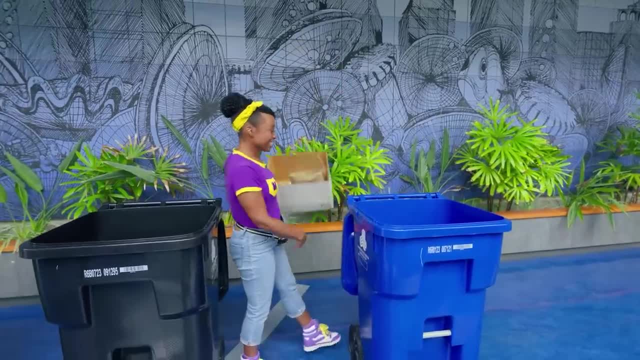 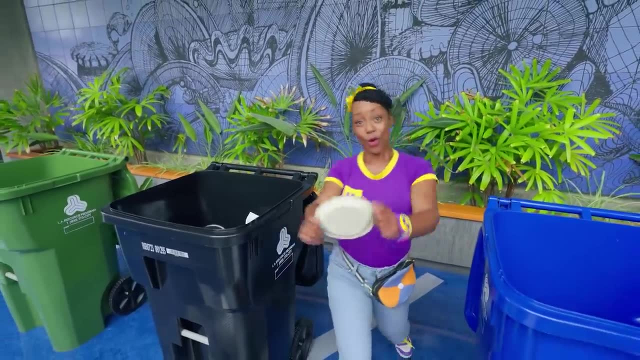 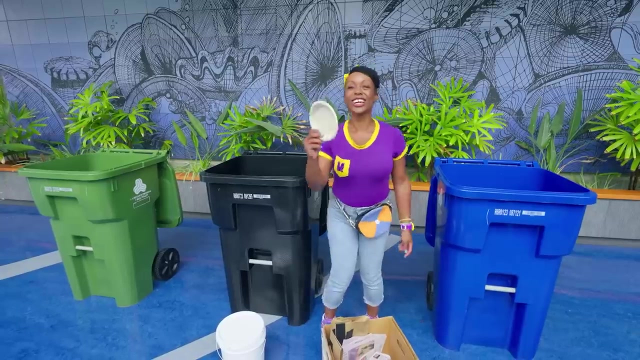 Maybe some orange juice. See ya, All right, What else? Oh, what about this? No, it's not a steering wheel, It's a plate. Do you know where it goes? Yes, we sort it with the compost. Okay, let's see if I can make it. 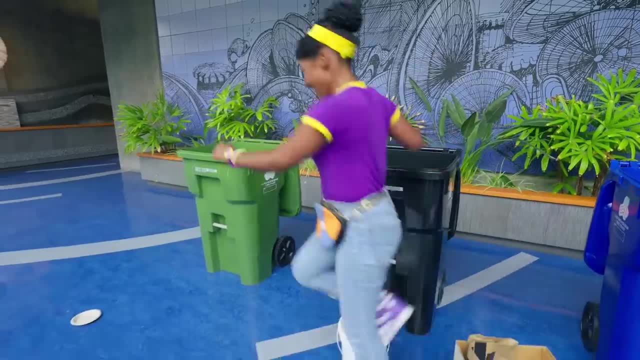 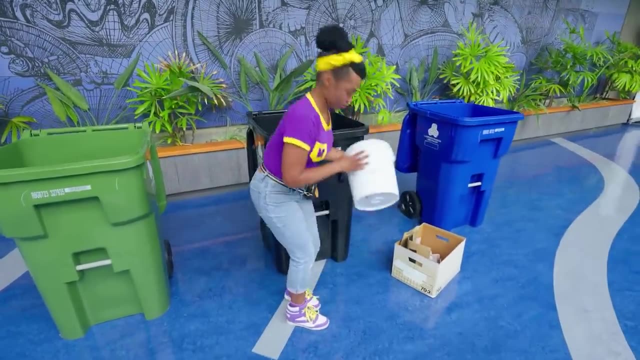 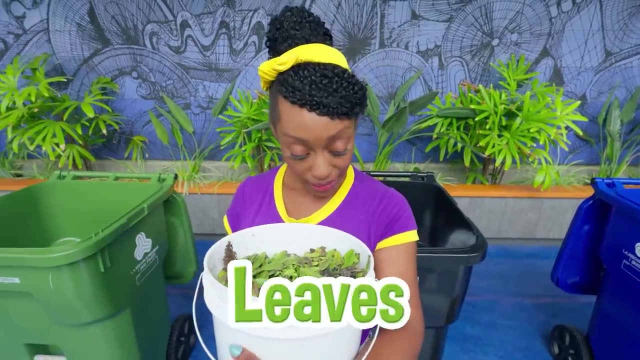 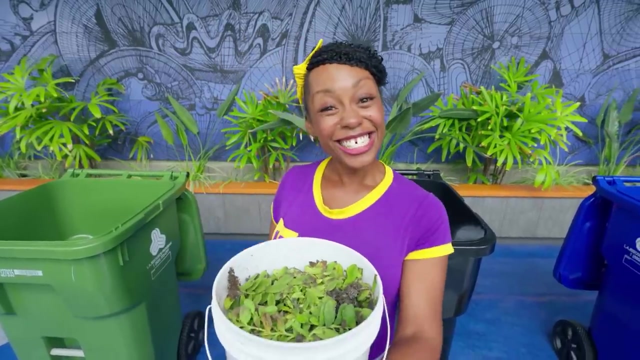 Frisbee. Okay, here you go. Woo Hey, where'd this come from? I wonder what's inside. Let's see. Oh, some leaves Yard waste. Do you know where yard waste goes? That's right Into the green compost bin. 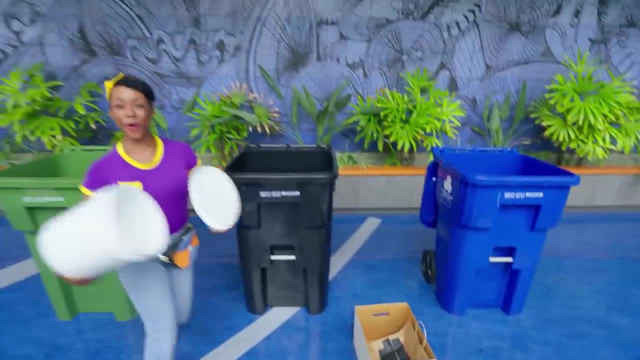 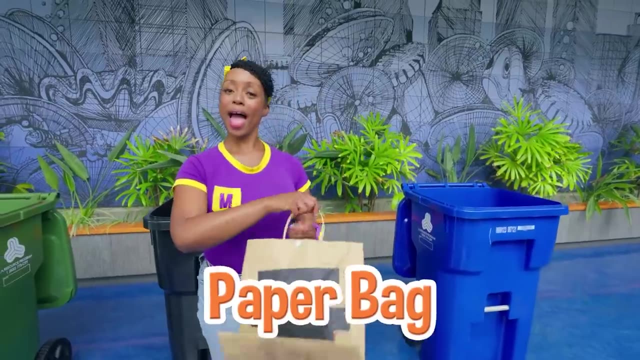 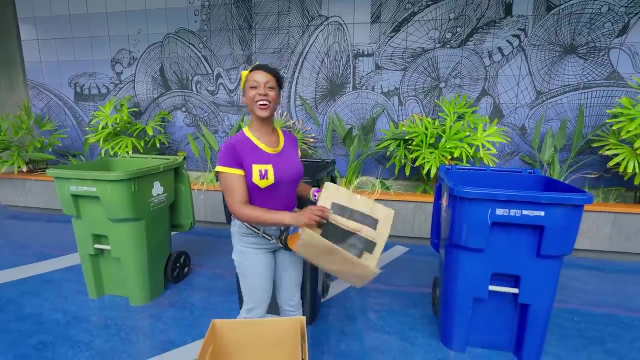 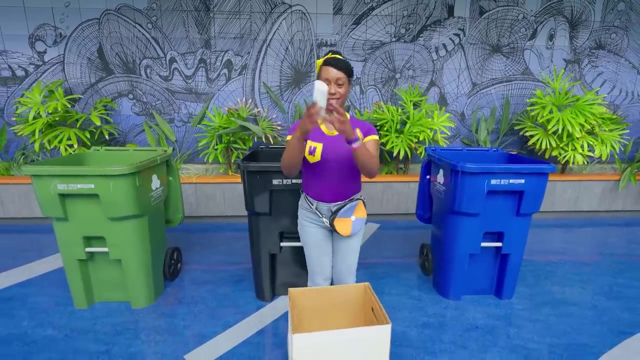 Woo, Oh, all right, Let's see what else we have to sort. Oh, check it out. A paper bag for shopping. Do you know where the paper bag goes? That is right, A paper goes into the recycling bin. Okay, one more thing in our box. 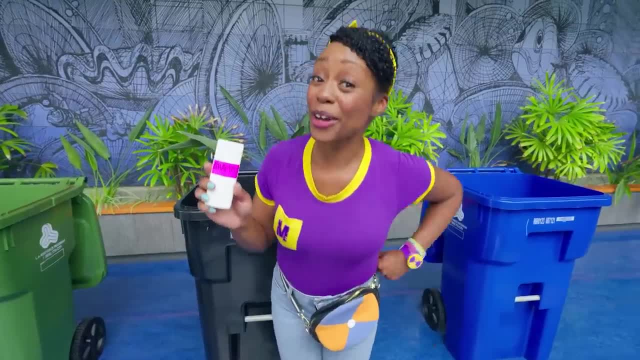 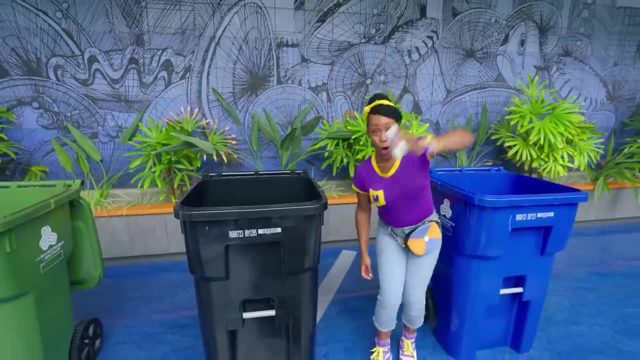 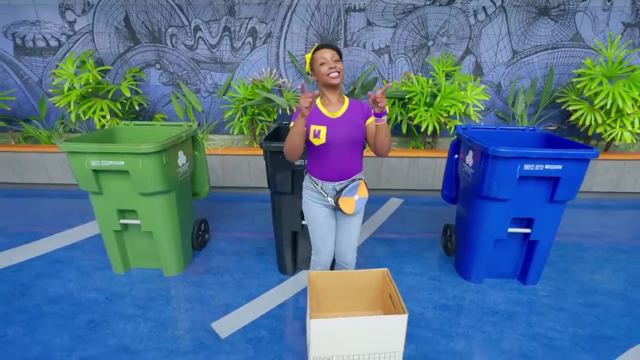 My shampoo bottle. Do you know where the shampoo bottle goes, Mm-hmm. After it's all cleaned out, it goes into recycling. Awesome, We sorted all our items. This calls for a 10.. Okay, Second, second wait. 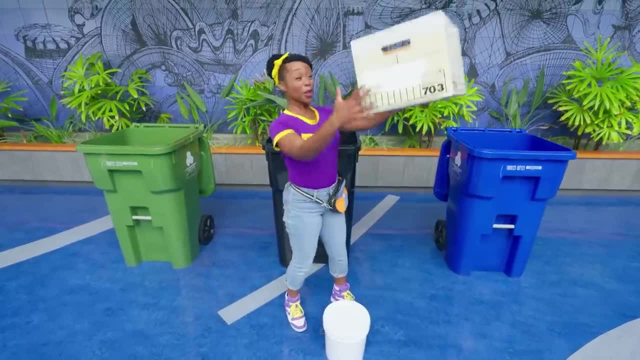 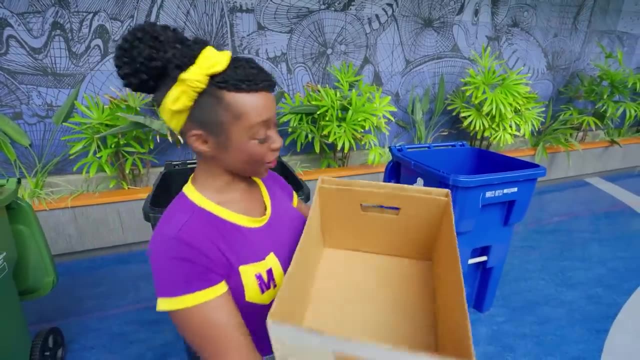 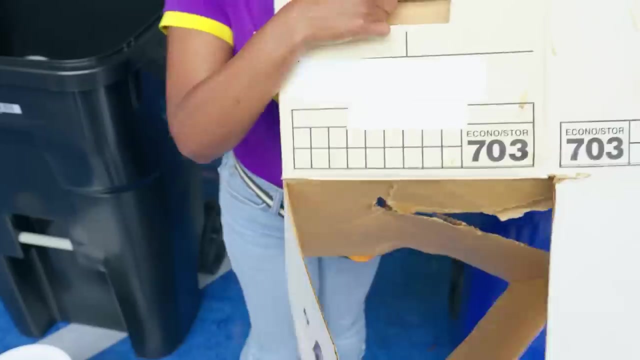 We forgot an item Mm-hmm: The cardboard box. Do you know where cardboard boxes go? That's right, They're paper. so they go into recycling, but only after you break it down. first, Break it down. Okay, Here you go. 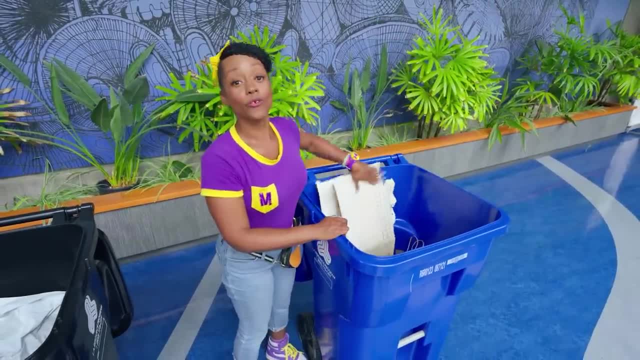 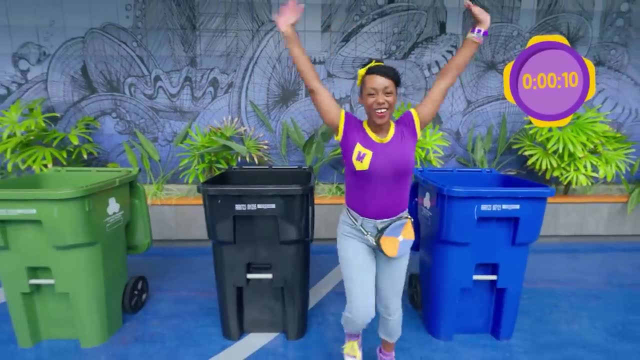 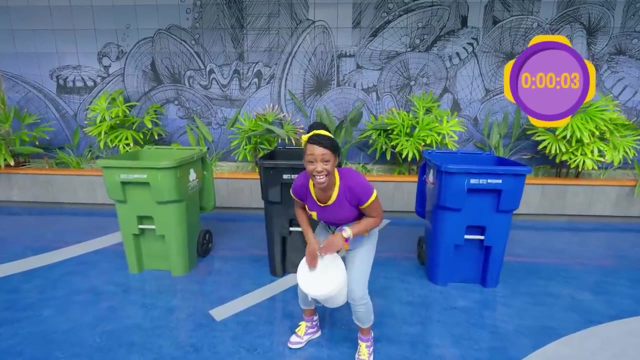 Into the recycling. Yeah, you have to break down the boxes so you have more room for more recycled tools. Okay, this calls for a 10 second dance party. We did it, we did it. We never ever quit it. We did it. that was so much fun. woo hoo. 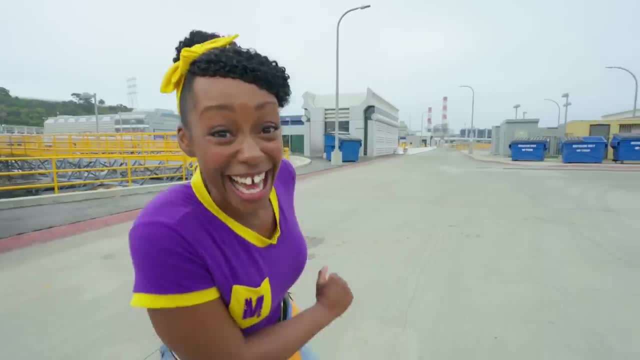 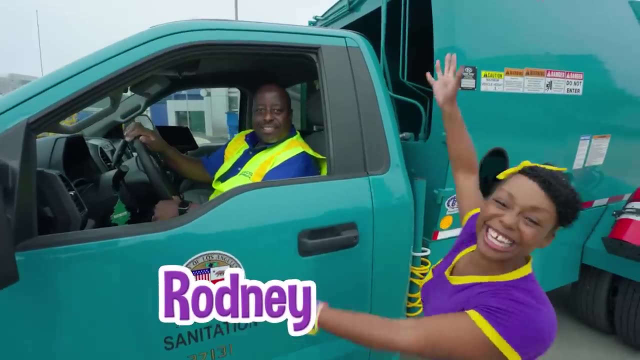 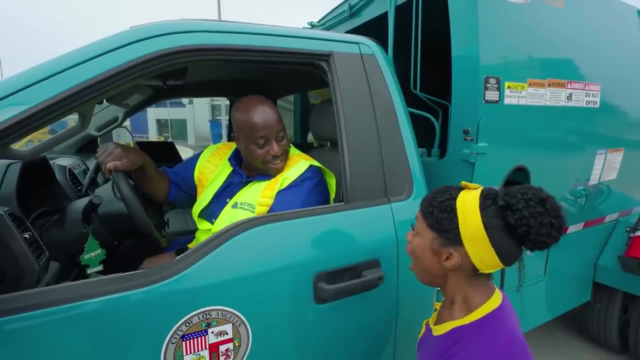 Oh, I want to introduce you to someone. Here he comes. This is my friend Rodney. Hello everyone, hello Mika, how are you Very well, Great, hey. would you like to go for a ride with me and I can show you how to pick up clean recycling. 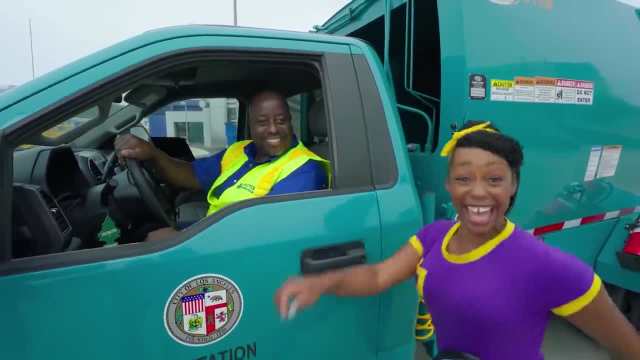 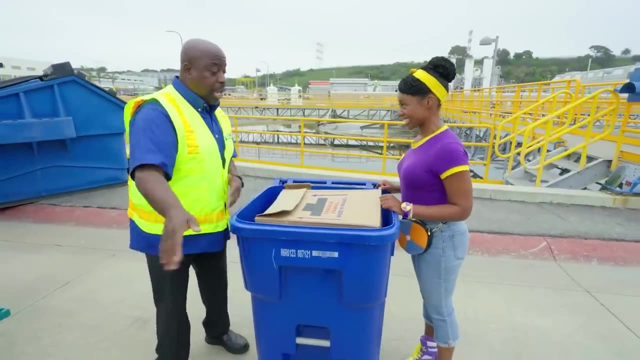 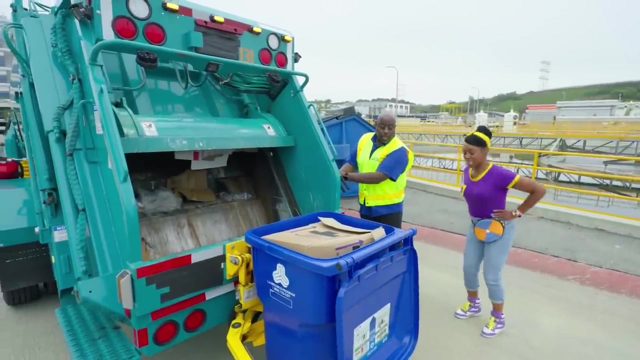 Oh, that sounds awesome. Great, come on, let's go. Okay, here I go. Okay, Mika, we'll put the can by Buster and have Buster eat it all up for us, Because Buster loves clean recycling. Oh yummy, it's time for some lunch, Buster. 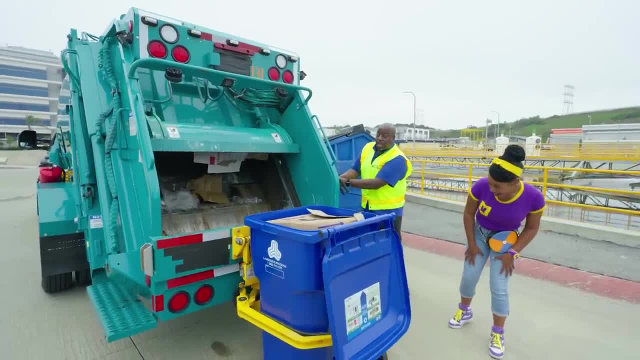 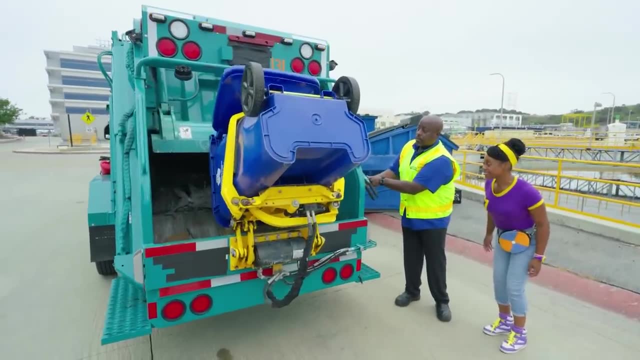 We grab it real gently with the grabbers. Buster has to do it. We have some nice little grabbers and we lift it up. Oh whoa, Yum, yum, yum. We have Buster eat it all up. I think he wants some seconds. 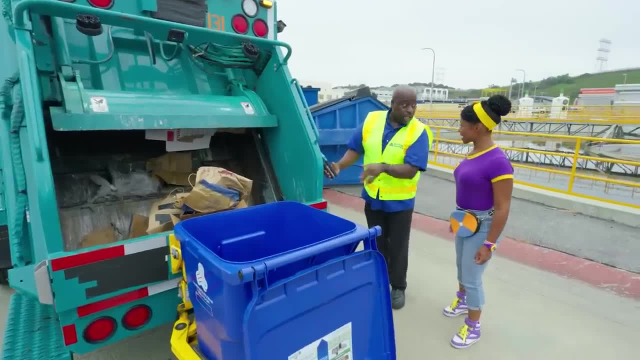 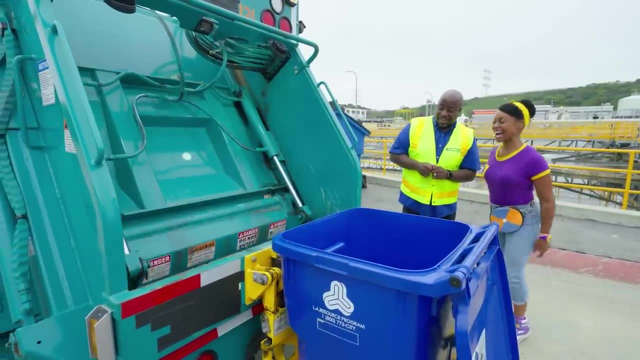 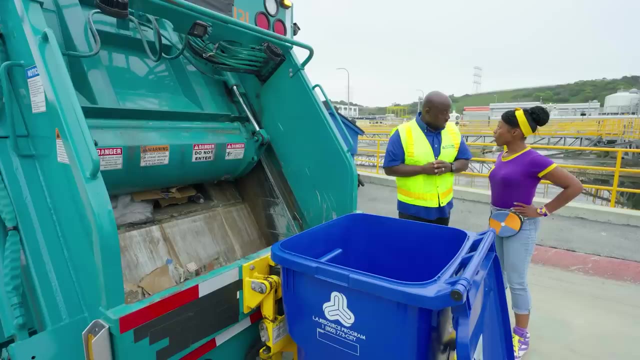 Yes, So this is what Buster does when he's really hungry for clean recycling: Whoa, Eat it all up, Buster, Tasty huh, There we go. Wow, And that's how we eat clean recycling. And Buster is satisfied with clean recycling.